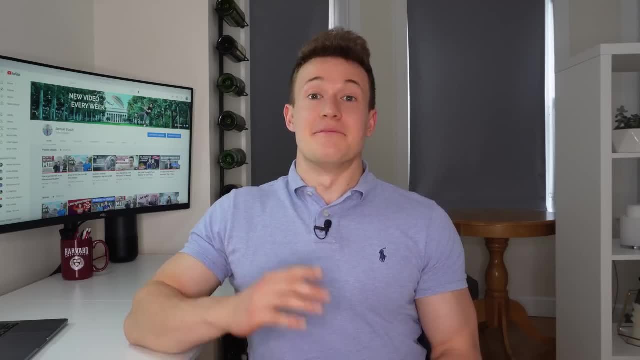 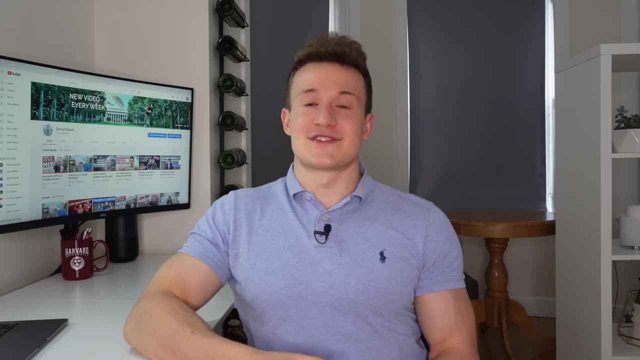 if you think you're bad at math, At the end of this video I'm going to give you the best resources to get you started on this journey, depending on your age and educational background. Brace yourself. I'm going to change the way you see numbers forever. 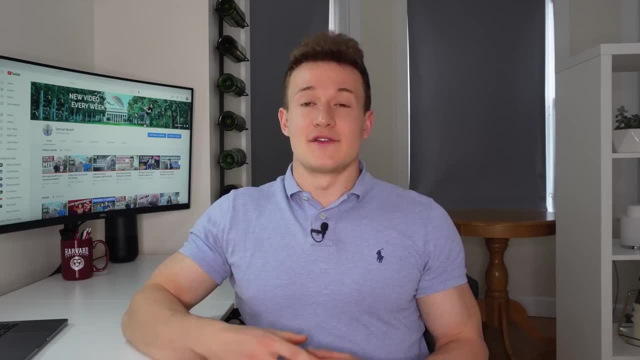 As I said, I used to be rather average at math. I used to do all of my homework problems and then maybe solve a few more problems before math exams and then I would perform okay in all of these exams. And sure, that approach kind of works if your goal is just being okay in all of 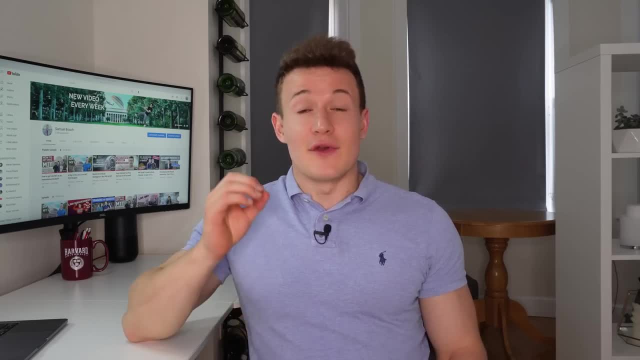 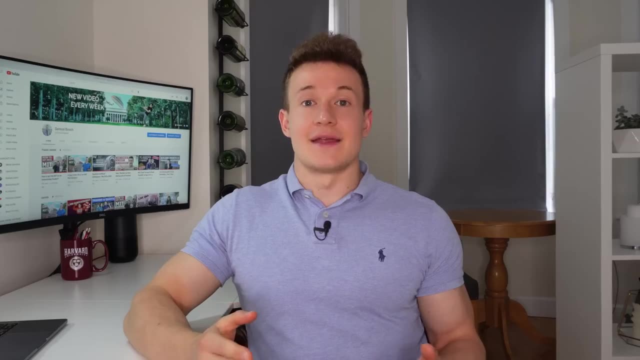 your exams. But the sad reality is that with this method, you will never become one of the people who can truly understand mathematics intuitively and who can utilize this potential in their daily lives. And don't fool yourself by thinking that only engineers and scientists use math on a day-to-day. 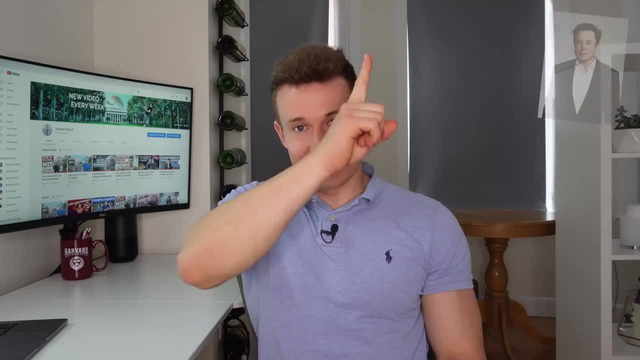 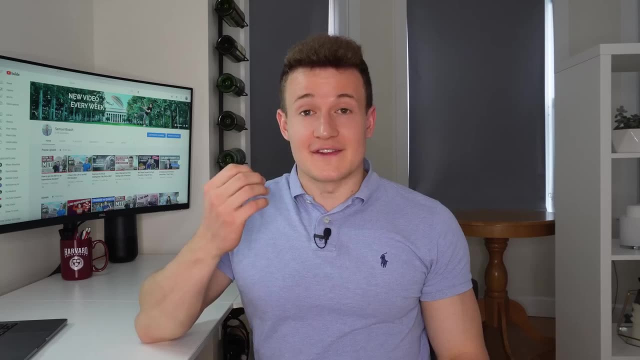 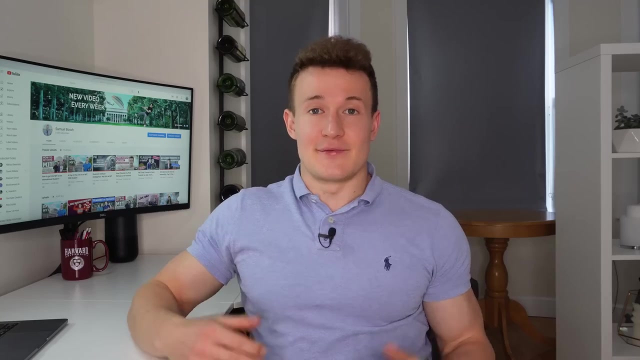 basis. Almost every successful person on this planet understands and uses math intuitively, Even without calculating anything explicitly. they can all make smart and intuitive decisions based on very good estimates of numbers, probabilities, risks and other factors. You probably think that I'm some kind of child genius. 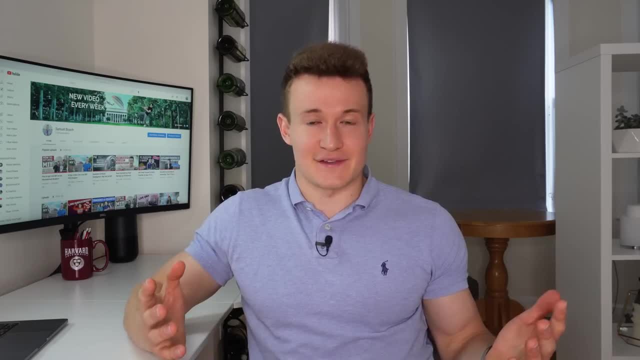 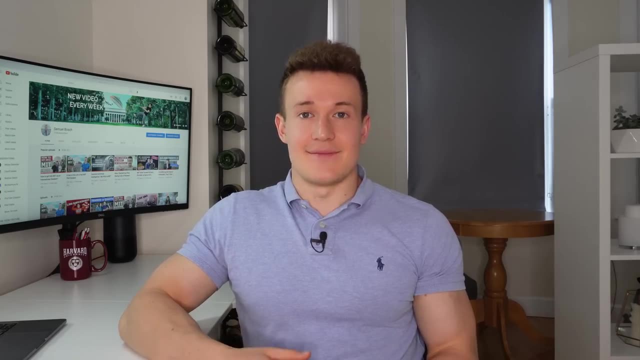 who just happened to become excellent in math and therefore got offered $50,000 a month for an internship. Well, this couldn't be further from truth. I would argue that understanding mathematics is 90% dependent on, first of all, your mindset, which I want to change in this video, and second, 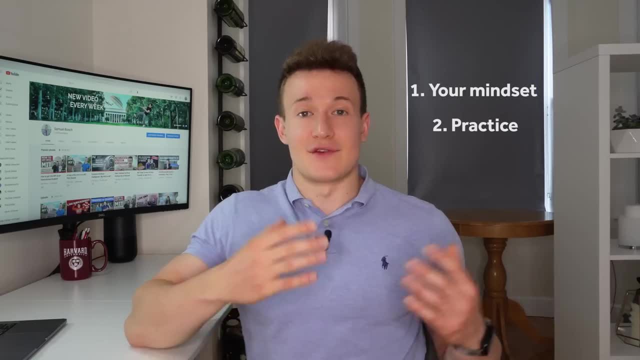 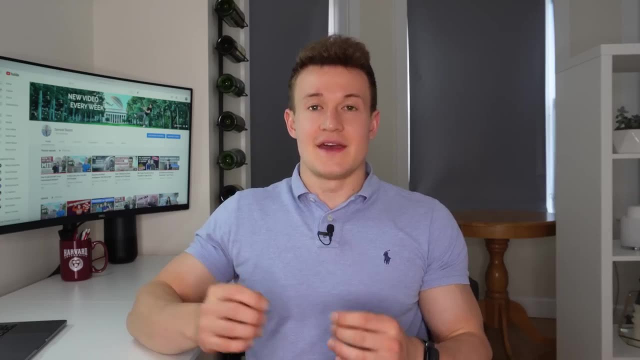 of all, lots and lots of problem-solving practice. using the right material, which I'm going to give you at the end of this video, Math can be understood intuitively, Contrary to history or geography, where you can only know the facts that you have actually learned. 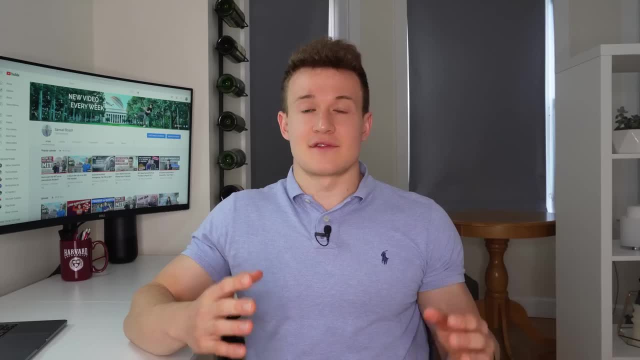 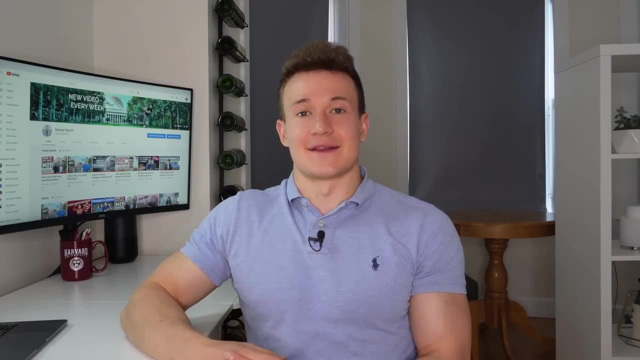 you can develop the ability to understand mathematics intuitively so that you can solve new problems that you have never encountered before. Let us now get to the main point of this video. How can you develop such mathematical intuition? Obviously, this doesn't happen overnight. If you have an exam in math tomorrow, 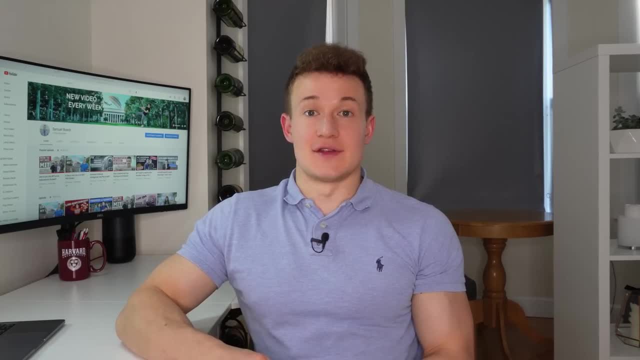 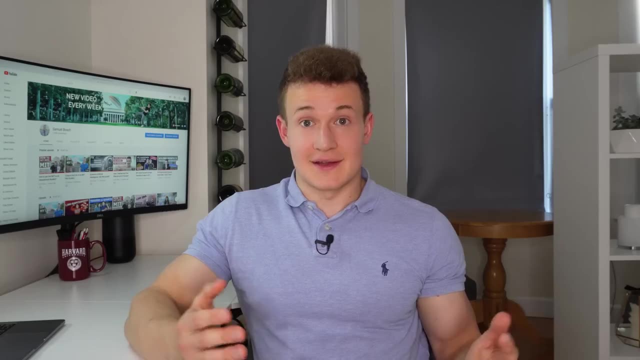 this video isn't going to save you. Instead, I want you to use this video as a start of a transformation that will take at least several weeks or months to show significant impact, But this may as well become the most valuable thing that you will ever learn. 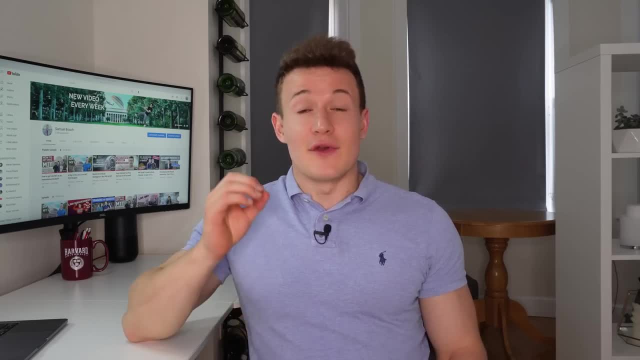 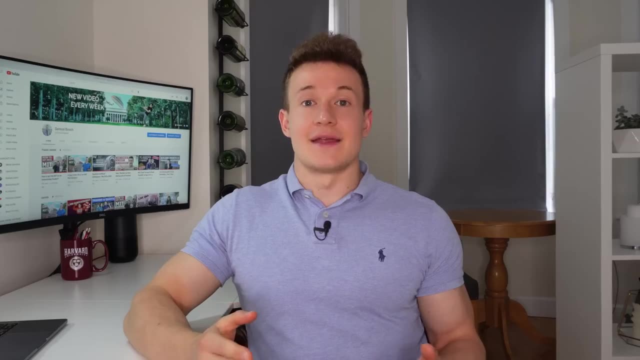 your exams. But the sad reality is that with this method, you will never become one of the people who can truly understand mathematics intuitively and who can utilize this potential in their daily lives. And don't fool yourself by thinking that only engineers and scientists use math on a day-to-day. 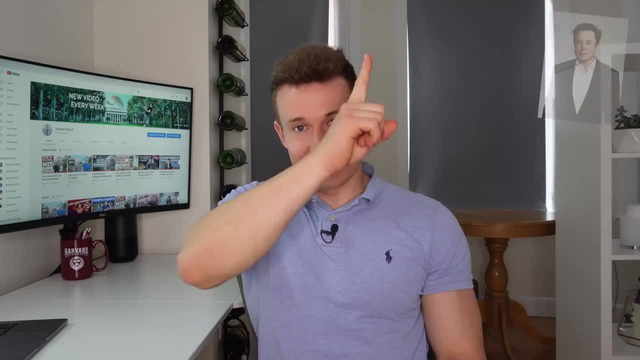 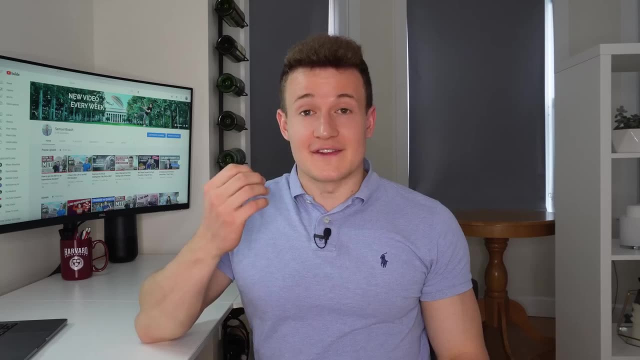 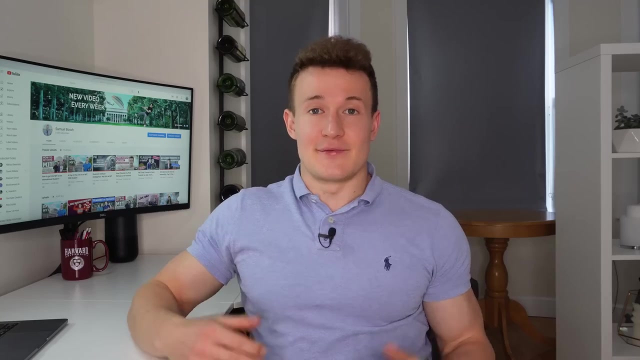 basis. Almost every successful person on this planet understands and uses math intuitively, Even without calculating anything explicitly. they can all make smart and intuitive decisions based on very good estimates of numbers, probabilities, risks and other factors. You probably think that I'm some kind of child genius. 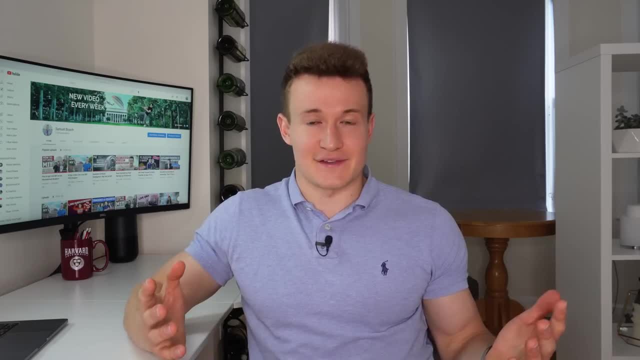 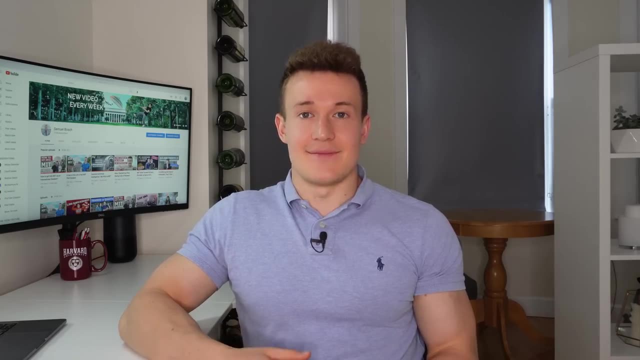 who just happened to become excellent in math and therefore got offered $50,000 a month for an internship. Well, this couldn't be further from truth. I would argue that understanding mathematics is 90% dependent on, first of all, your mindset, which I want to change in this video, and second, 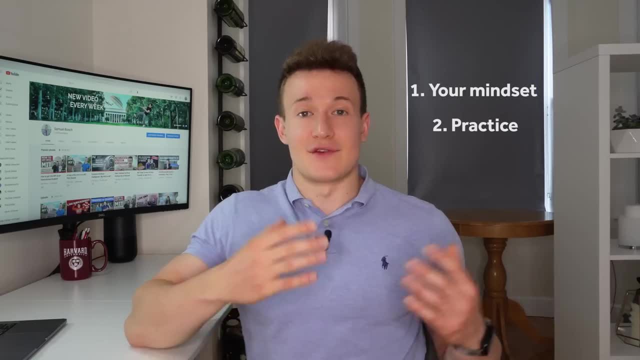 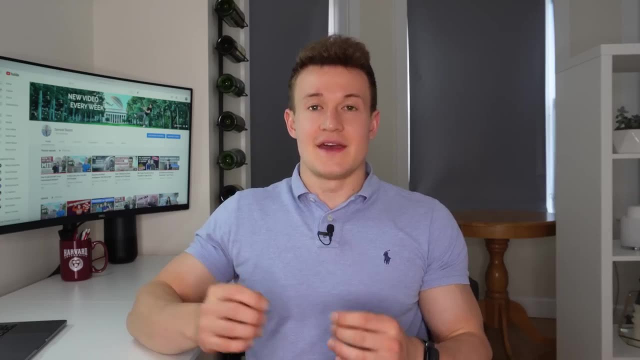 of all, lots and lots of problem-solving practice. using the right material, which I'm going to give you at the end of this video, Math can be understood intuitively, Contrary to history or geography, where you can only know the facts that you have actually learned. 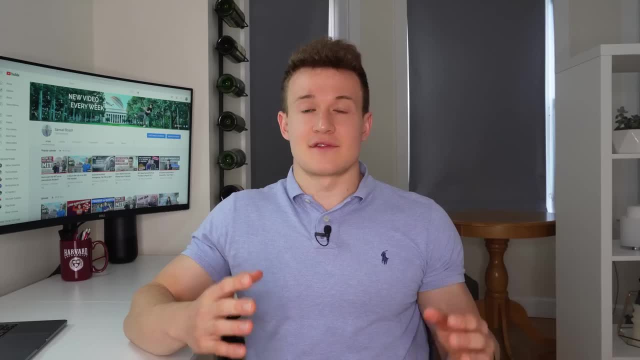 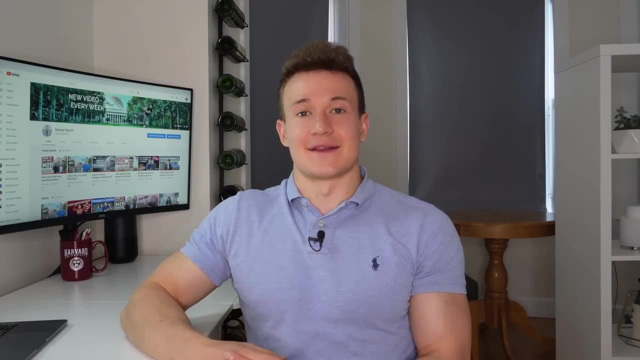 you can develop the ability to understand mathematics intuitively so that you can solve new problems that you have never encountered before. Let us now get to the main point of this video. How can you develop such mathematical intuition? Obviously, this doesn't happen overnight. If you have an exam in math tomorrow, 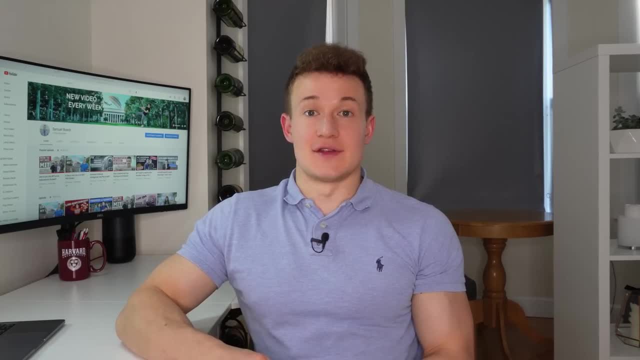 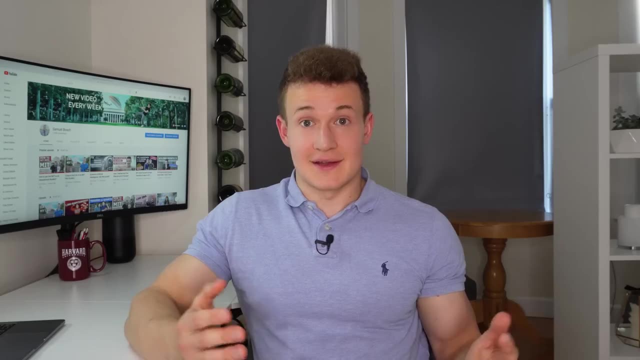 this video isn't going to save you. Instead, I want you to use this video as a start of a transformation that will take at least several weeks or months to show significant impact, But this may as well become the most valuable thing that you will ever learn. 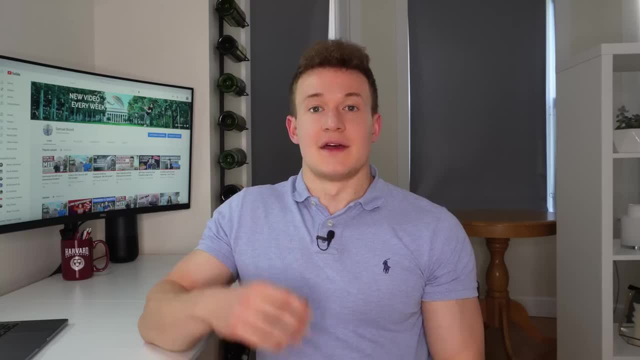 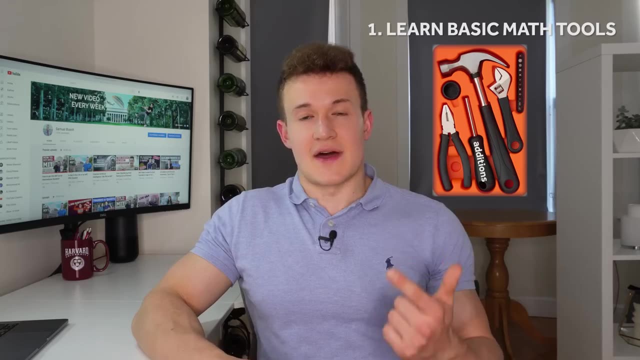 The way to develop a great mathematical intuition is the following. The first step is make sure to at least learn the basic concepts. Think about them as tools in your toolbox: Additions, fractions, decimal numbers. these are your basic tools. They are the hammers, wrenches and 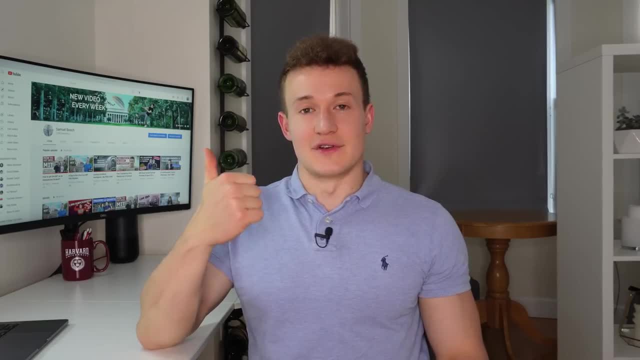 brackets. Every time you learn a new chapter in school, you add one tool to your toolbox And by the time you graduate from high school or university, you have accumulated an enormous amount of tools that are most likely just rusting in your basement. Time to wipe off the dust and put 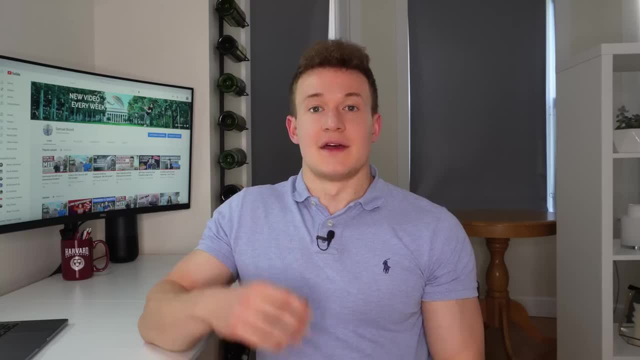 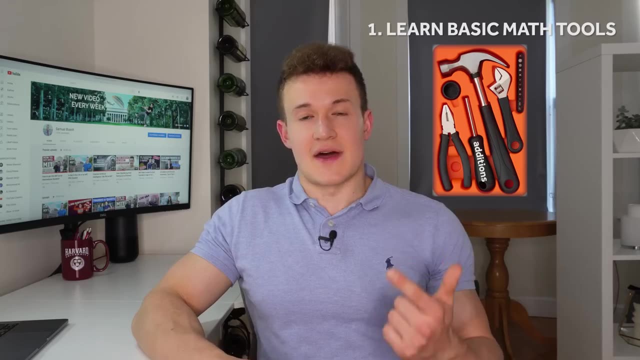 The way to develop a great mathematical intuition is the following. The first step is make sure to at least learn the basic concepts. Think about them as tools in your toolbox: Additions, fractions, decimal numbers. these are your basic tools. They are the hammers, wrenches and 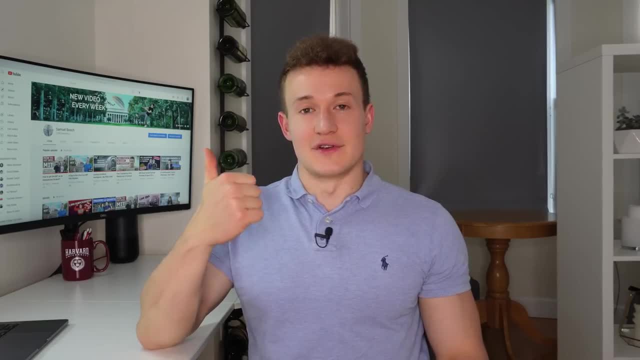 brackets. Every time you learn a new chapter in school, you add one tool to your toolbox And by the time you graduate from high school or university, you have accumulated an enormous amount of tools that are most likely just rusting in your basement. Time to wipe off the dust and put 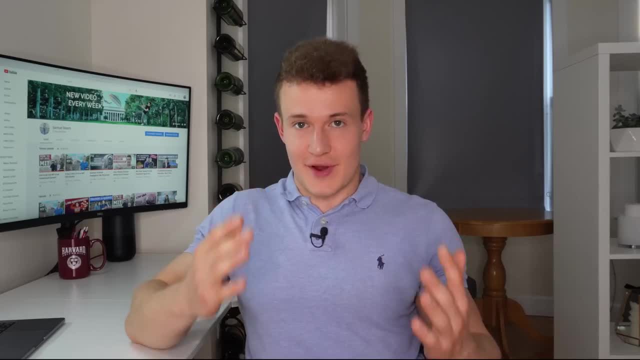 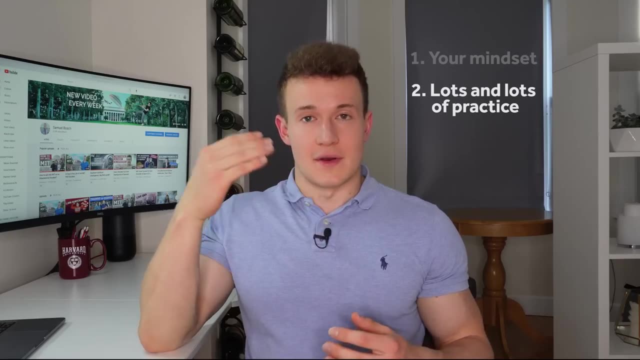 them to use in step number two. The next step is an enormous amount of problem-solving practice using the right materials that I will provide to you in a bit. Instead of just studying for an exam and then moving on to learning the next tool, you should stick to your simple toolbox initially. 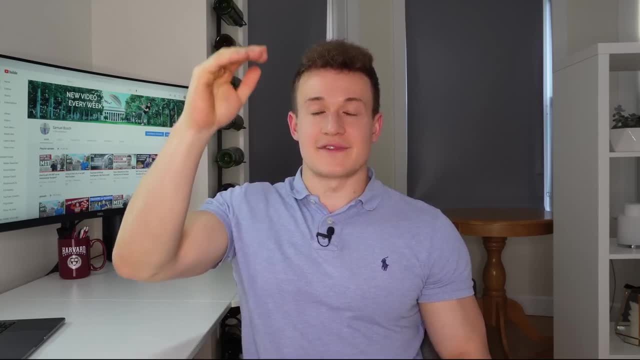 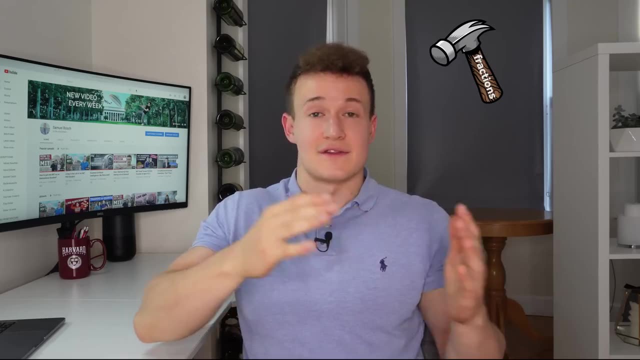 start with simple problems and then move on to learning the next tool And then work your way up to very hard problems using these exact same simple tools. You would be very surprised how advanced problems can be solved using just a hammer and a screwdriver. 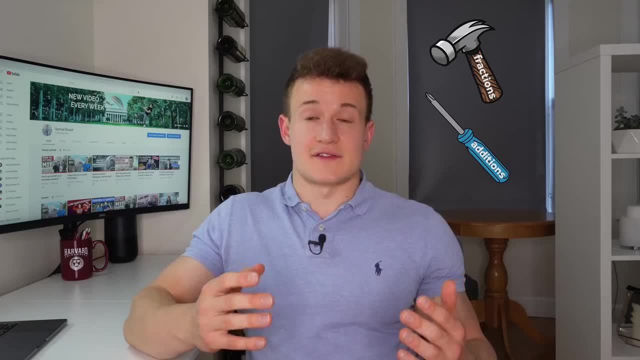 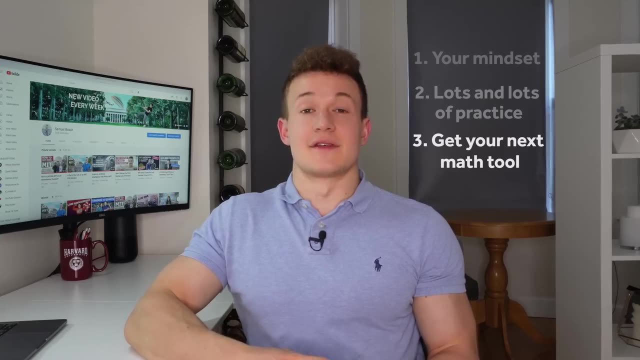 of mathematics. The third step, after you have really exhausted all the tools in your toolbox, is going on and adding a new tool to your toolbox. The problem with most education systems in the world is that this step happens way too early. Typically, you have just barely learned how to. 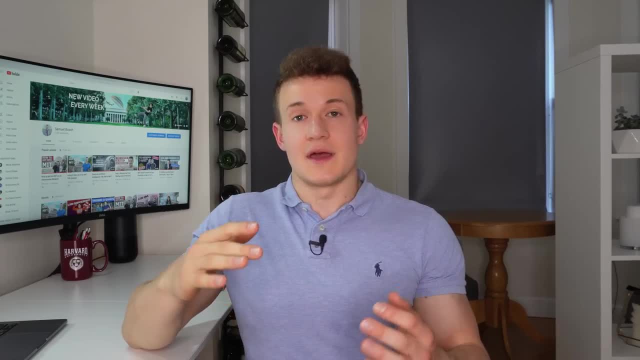 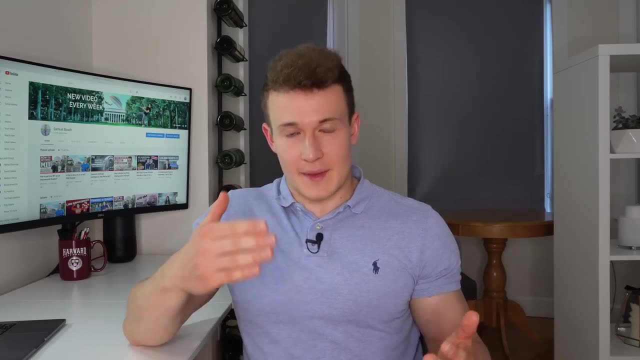 solve like three or five different types of problems using a given tool. Then you move on to the next one, And the word learn may be an overstatement here, because many students just memorize the steps to solving a problem and then just repeat the same thing during an exam. 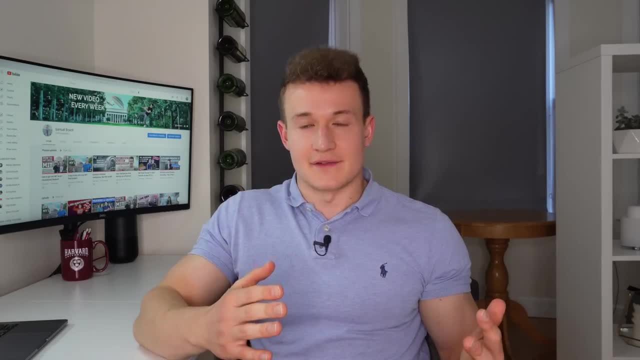 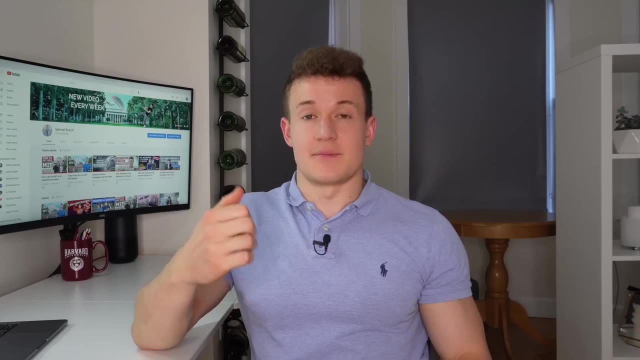 but with different numbers. Most school systems are set up to value good memorizers who can reproduce what teachers showed them and push away those creative, deep thinkers. As a rule of thumb, for every one hour that you spend learning a new tool, you should spend at least 20 to 100 hours. 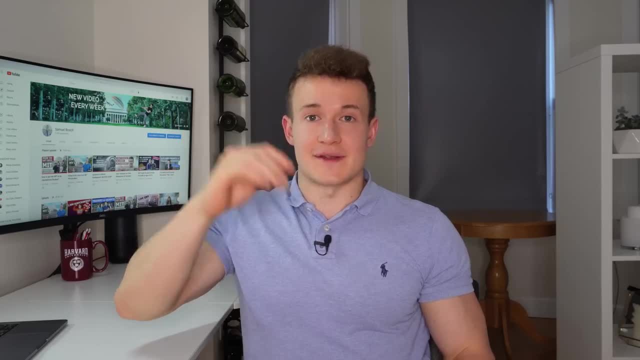 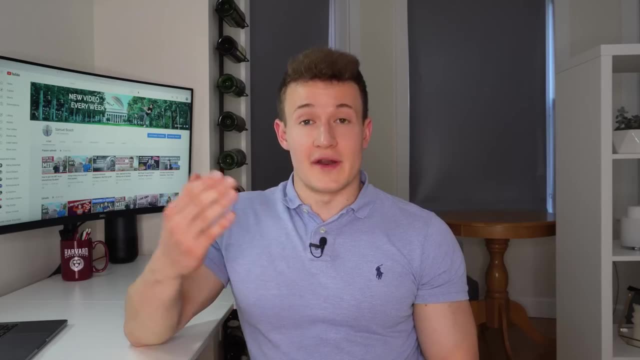 practicing using these tools, first on simple and then very advanced mathematical problems. Alright, you've made it this far in the video. Now you have to make a big decision. Do you want to forever change your academic and professional life by learning to understand math? 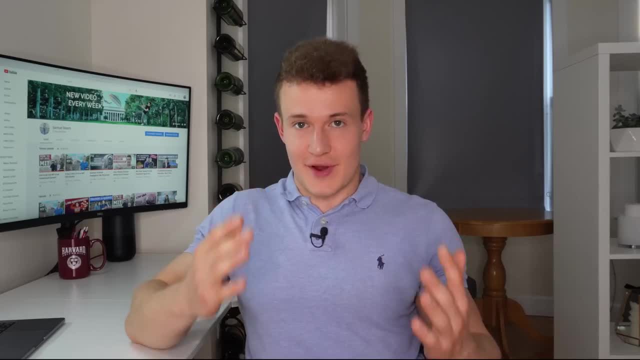 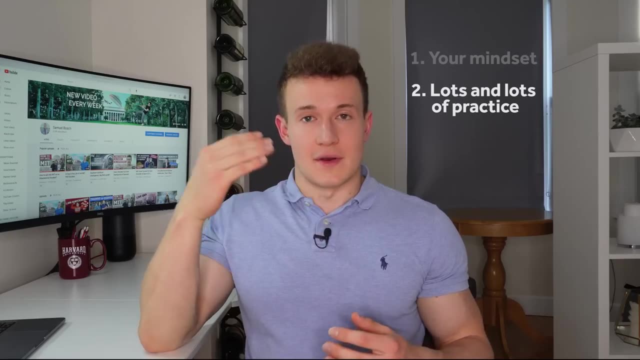 them to use in step number two. The next step is an enormous amount of problem-solving practice using the right materials that I will provide to you in a bit. Instead of just studying for an exam and then moving on to learning the next tool, you should stick to your simple toolbox initially. 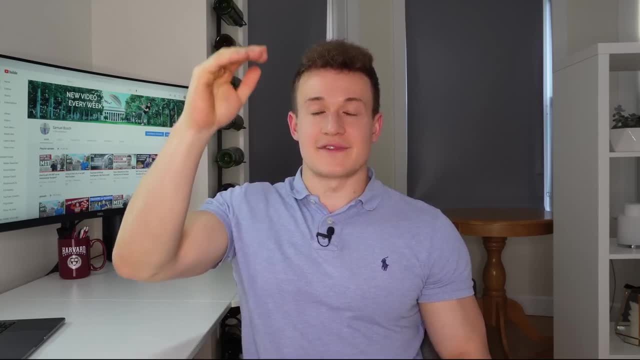 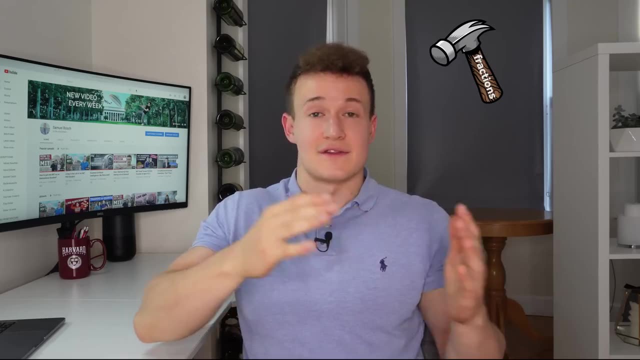 start with simple problems and then move on to learning the next tool And then work your way up to very hard problems using these exact same simple tools. You would be very surprised how advanced problems can be solved using just a hammer and a screwdriver. 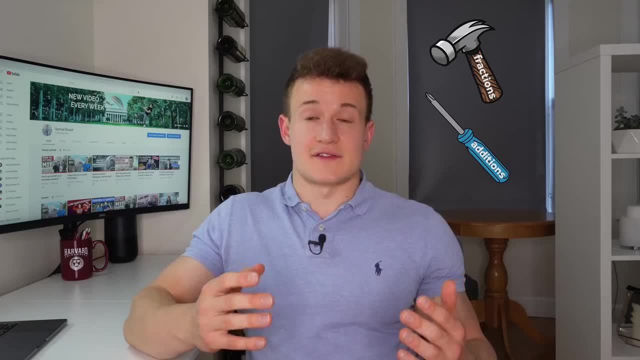 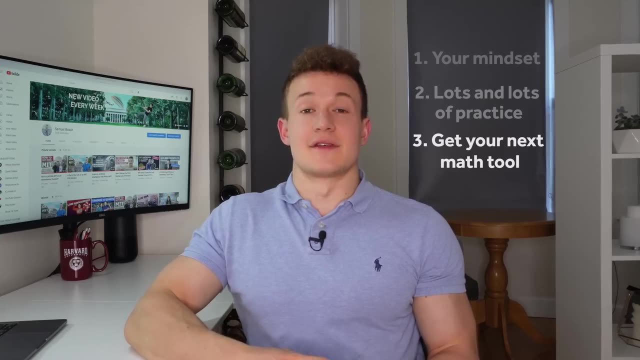 of mathematics. The third step, after you have really exhausted all the tools in your toolbox, is going on and adding a new tool to your toolbox. The problem with most education systems in the world is that this step happens way too early. Typically, you have just barely learned how to. 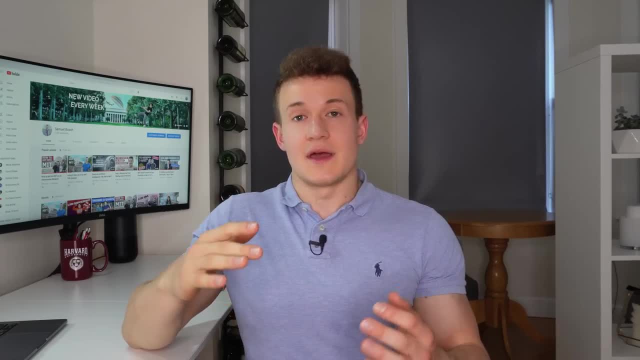 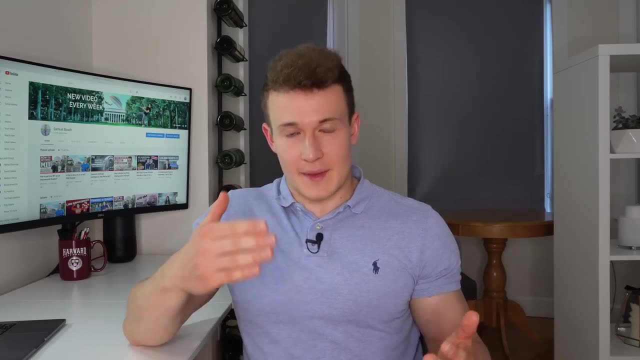 solve like three or five different types of problems using a given tool. Then you move on to the next one, And the word learn may be an overstatement here, because many students just memorize the steps to solving a problem and then just repeat the same thing during an exam. 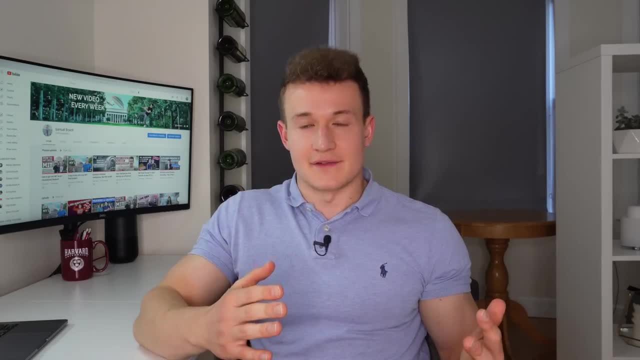 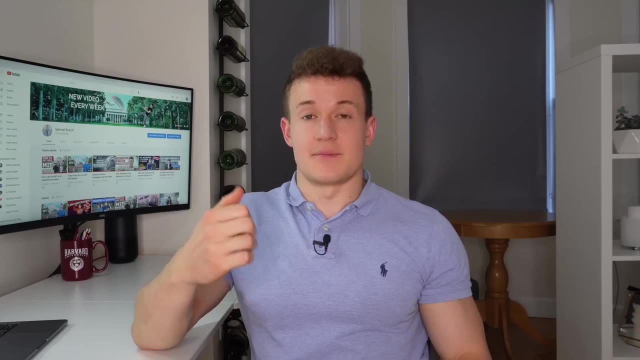 but with different numbers. Most school systems are set up to value good memorizers who can reproduce what teachers showed them and push away those creative, deep thinkers. As a rule of thumb, for every one hour that you spend learning a new tool, you should spend at least 20 to 100 hours. 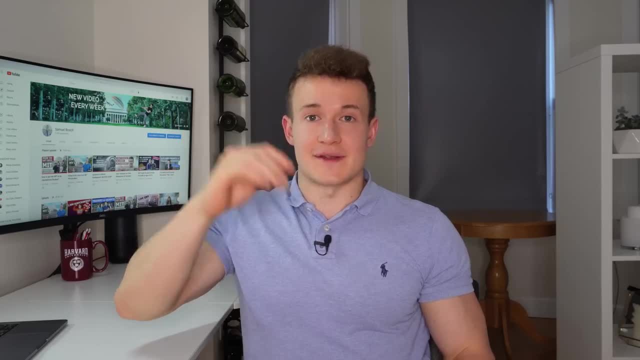 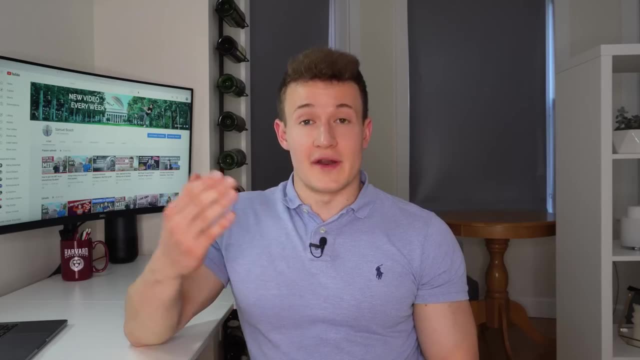 practicing using these tools, first on simple and then very advanced mathematical problems. Alright, you've made it this far in the video. Now you have to make a big decision. Do you want to forever change your academic and professional life by learning to understand math? 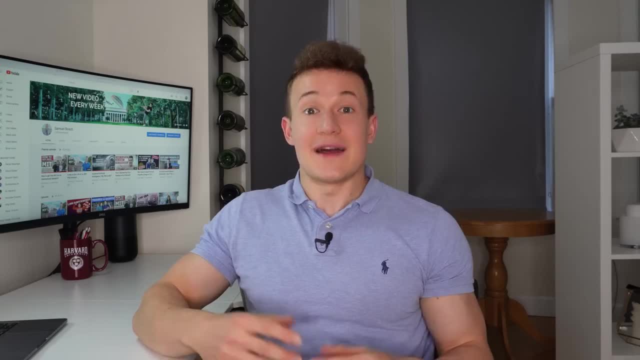 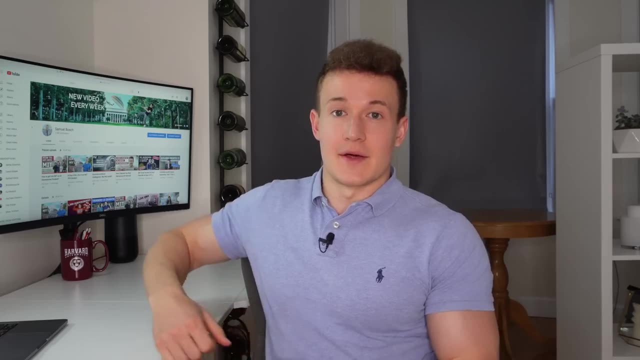 intuitively. If you decided yes, I will now give you the right resources to get you started, depending on your age and educational background. The most comprehensive set of resources is available on the website called wwwartofproblemsolvingcom, When you open their. 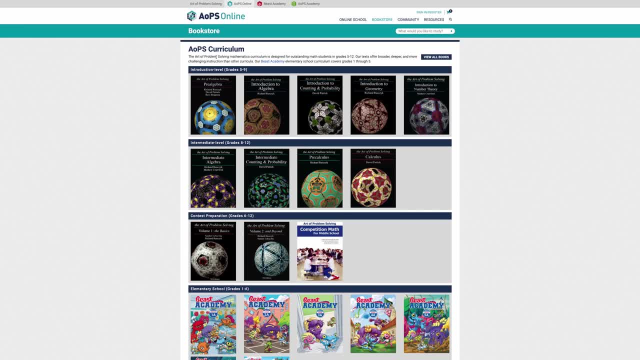 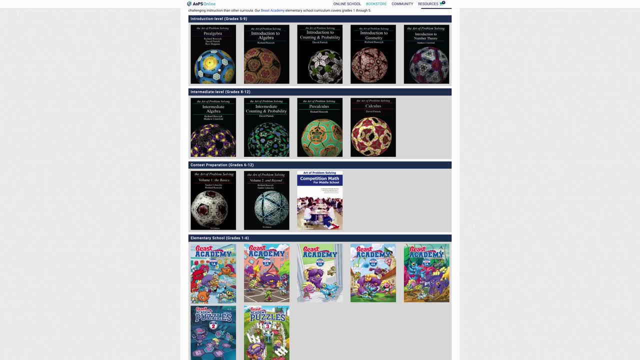 website you will find a complete set of resources ranging from elementary school, middle school, high school and early college. Don't be too focused on the year number, because these are rather advanced problems. So, for example, if you're in the last year of high school. 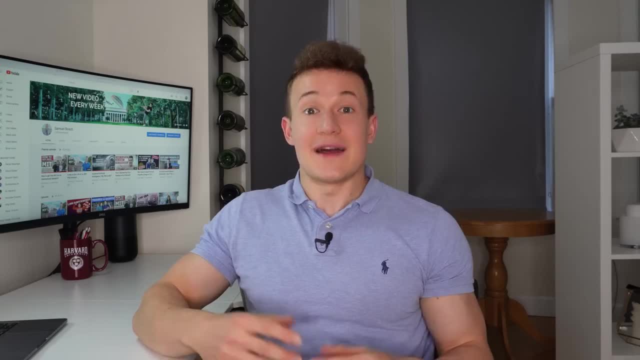 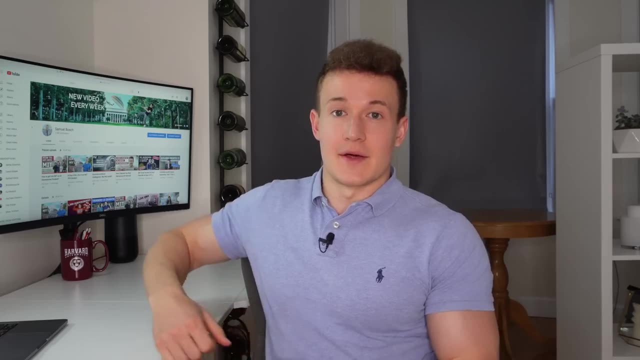 intuitively. If you decided yes, I will now give you the right resources to get you started, depending on your age and educational background. The most comprehensive set of resources is available on the website called wwwartofproblemsolvingcom, When you open their. 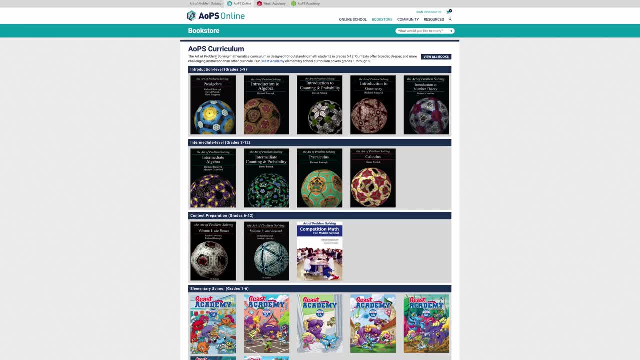 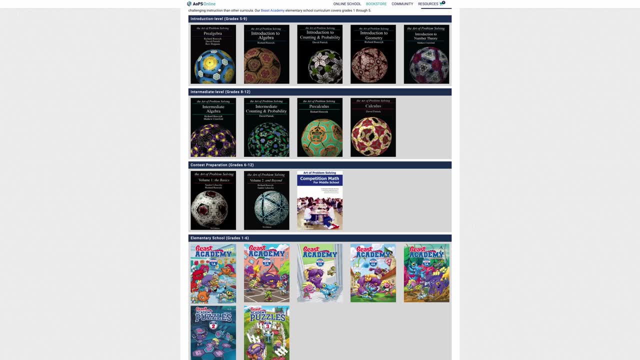 website you will find a complete set of resources ranging from elementary school, middle school, high school and early college. Don't be too focused on the year number, because these are rather advanced problems. so, for example, if you are in the last year of high school, you don't. 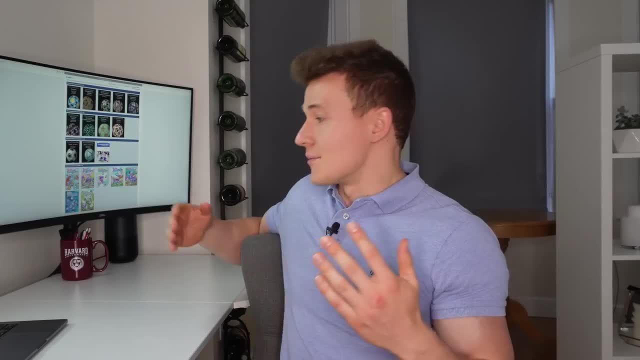 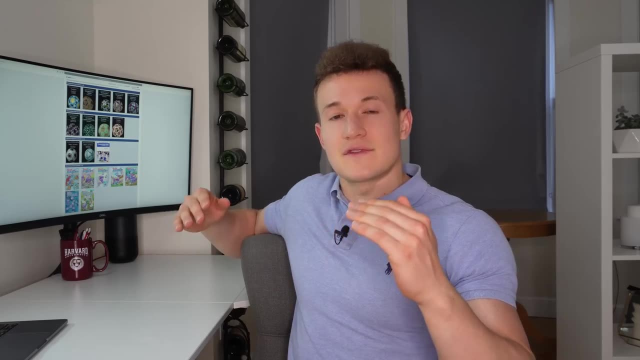 have to start necessarily with grade 12.. You may want to start with something a bit earlier and then work your way up. Remember, it's all about the toolbox and you want to start with simple problems and then use that same toolbox to learn how to solve advanced problems. 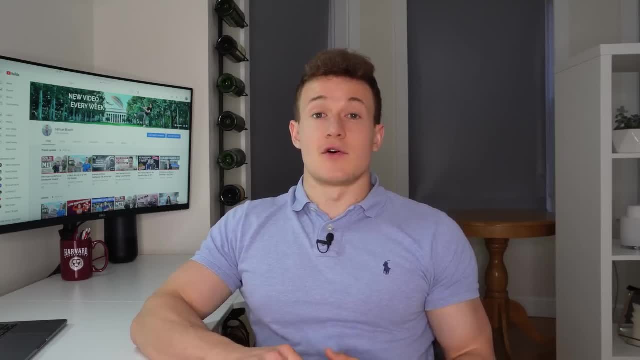 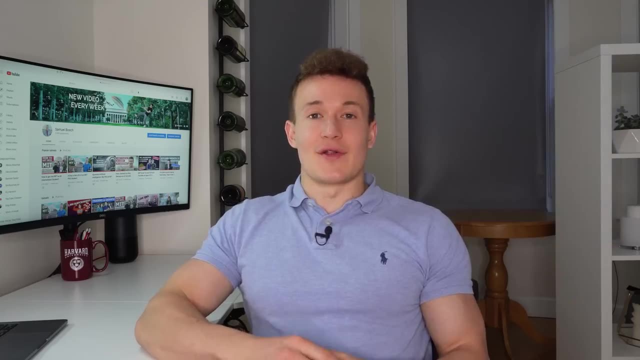 Speaking of simple toolboxes, another great book to get you started is called A Concise Introduction to Pure Mathematics by Martin Liebeck. Also, if you happen to speak German, there is a great book called Mathe is Cool, which is for everyone of 12 and over. If your toolbox already contains somewhat more advanced, 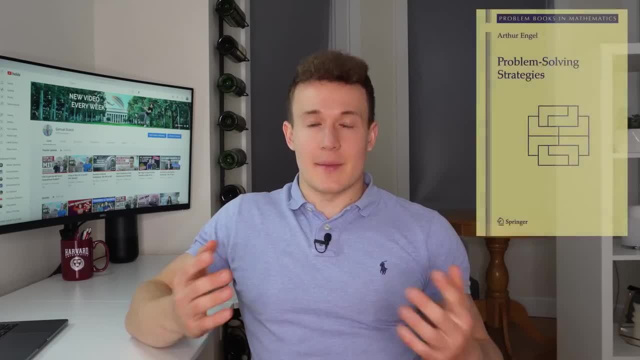 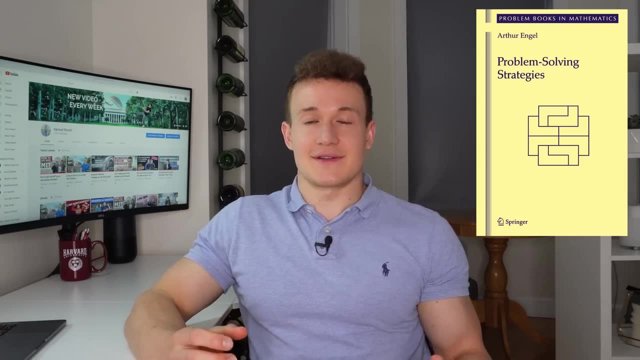 high school level tools, then you might want to have a look at a book called Problem Solving Strategies by Arthur Engel. This book is a collection of problems from many national and international math competitions and it contains very good resources and guides on how to tackle. 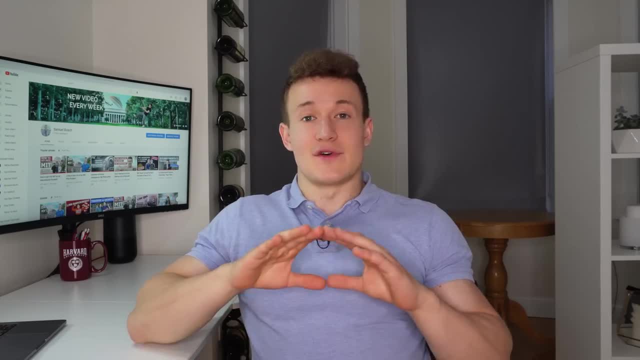 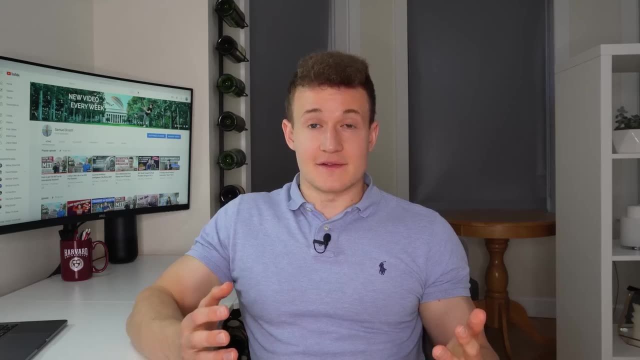 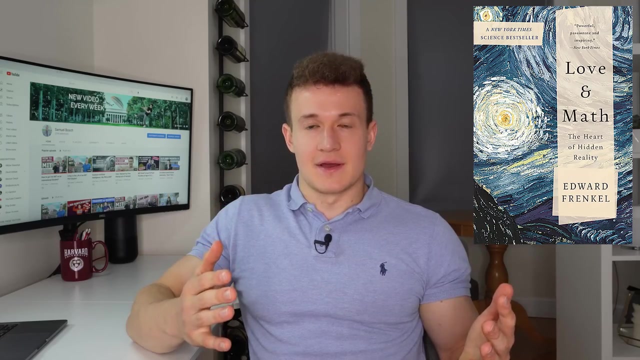 these problems in the first place. Also, I know a guy who solved all of these problems in the international math olympiad. For more mature audiences, I would also recommend the book Love and Math, The Heart of Hidden Reality by Edvard Frankl. It's not just a math textbook. 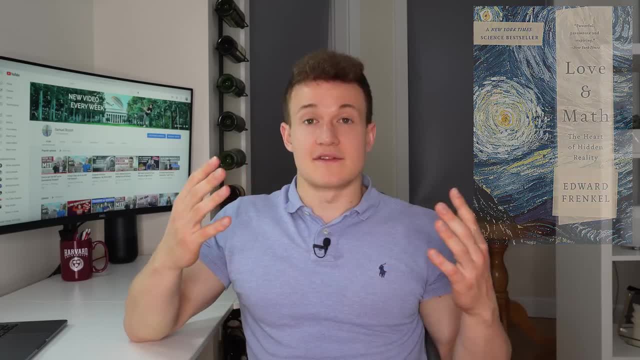 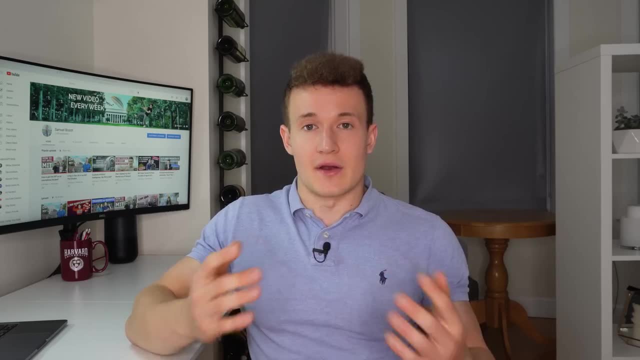 but it also talks about the beauty of mathematics and how to understand it and see it in a different way. Becoming good at math is in some way like becoming a good car mechanic. For sure, at some point you will have to acquire a lot of tools to do your job well, but a professional mechanic- 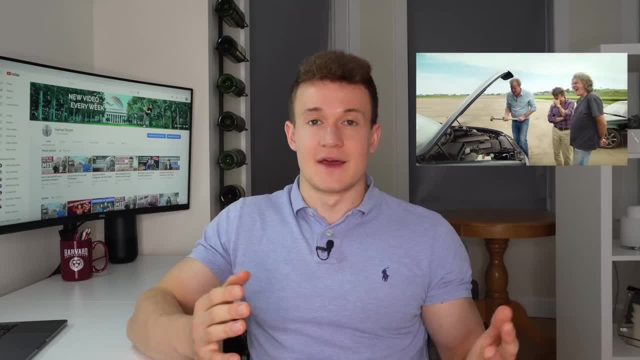 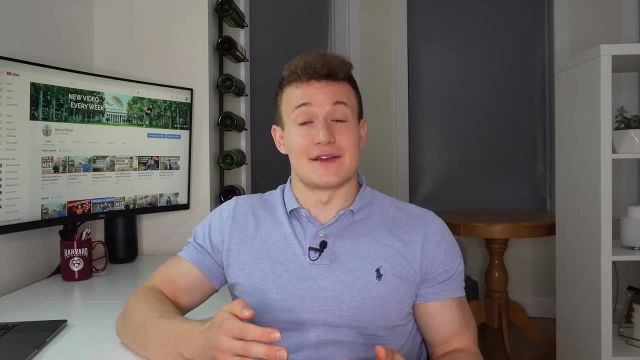 would be able to fix more cars with a $20 toolbox from Amazon than I would be able to do with a $100,000 mechanic shop. If you want to learn more about how to fix a car with a $100,000 toolbox, let me give you an open-ended question that captures the essence of mathematical intuition. 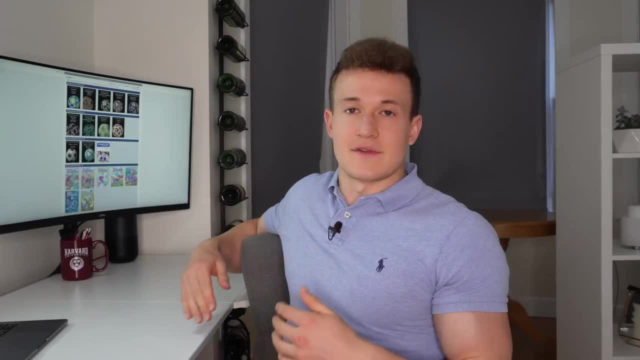 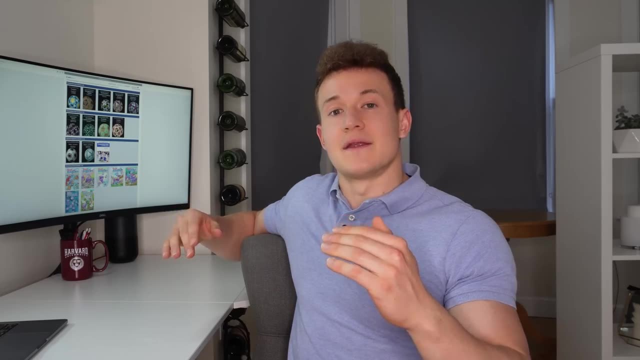 you don't have to start necessarily with grade 12.. You may want to start with something a bit earlier and then work your way up. Remember, it's all about the toolbox and you want to start with simple problems and then use that same toolbox to learn how to solve advanced problems. 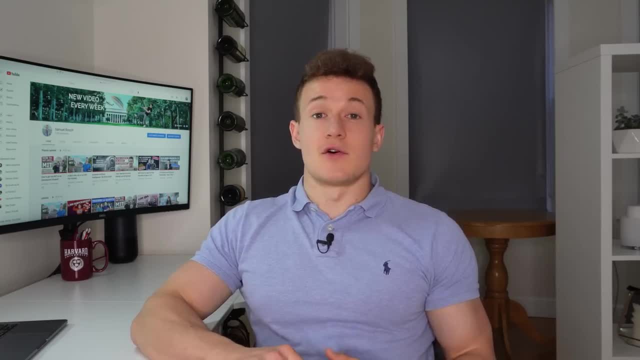 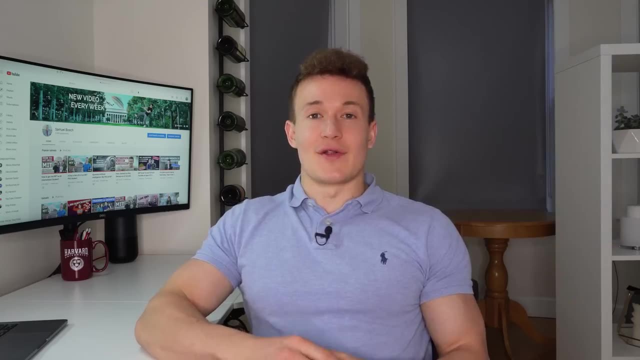 Speaking of simple toolboxes, another great book to get you started is called A Concise Introduction to Pure Mathematics by Martin Liebeck. Also, if you happen to speak German, there's a great book called Mathe is Cool, which is for everyone of 12 and over, If your toolbox already contains somewhat more advanced high school level tools. 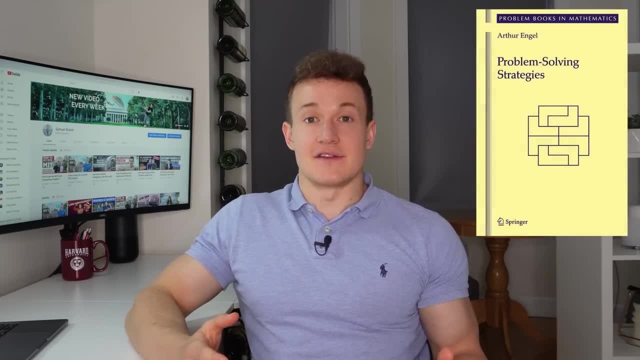 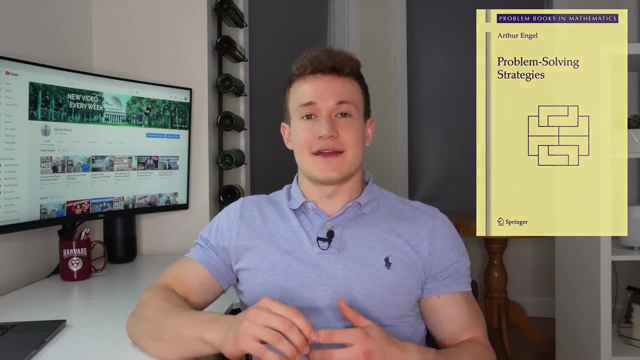 then you might want to have a look at a book called Problem Solving Strategies by Arthur Engel. This book is a collection of problems from many national and international math competitions, and it contains very good resources and guides on how to tackle these problems in the first place. 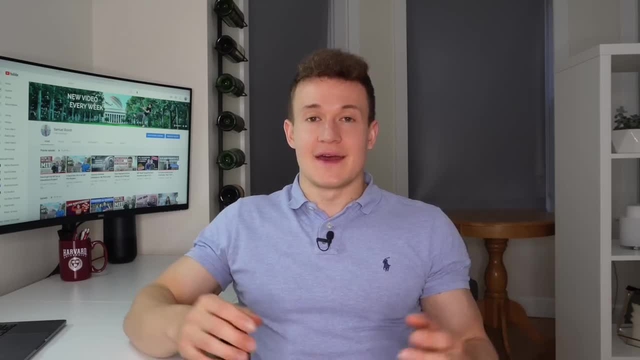 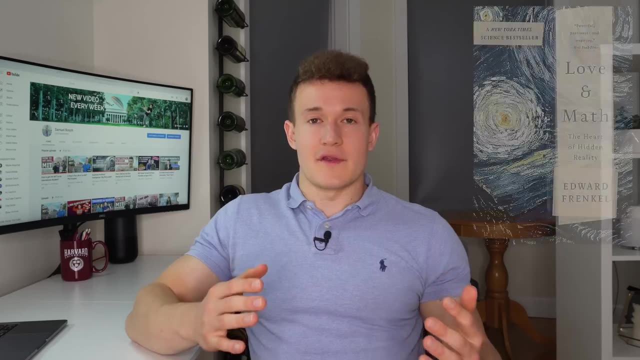 Also, I know a guy who solved all of these problems in the whole book and he ended up winning the International Math Olympiad. For more mature audiences, I would also recommend the book Love and Math- The Heart of Hidden Reality by Edvard Frankl. It's not just a math textbook, but it also. 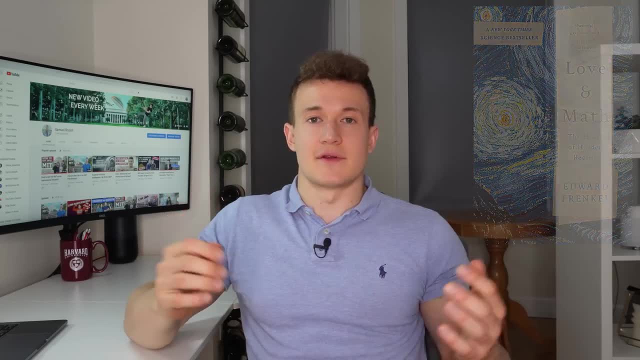 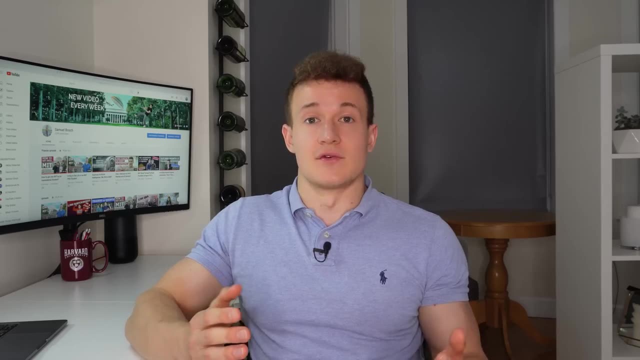 talks about the beauty of mathematics and how to understand it and see it in a different way. Becoming good at math is in some way like becoming a good car mechanic. For sure, at some point you will have to acquire a lot of tools to do your job well, but a professional mechanic would be able to. 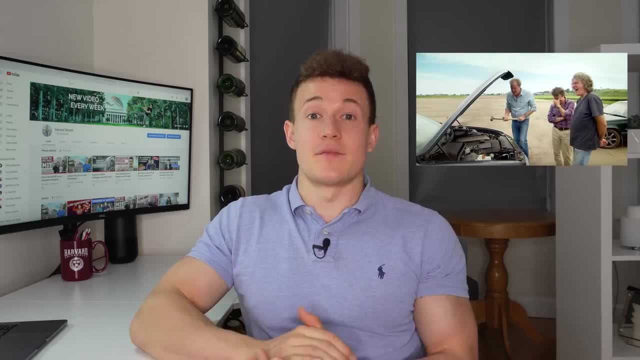 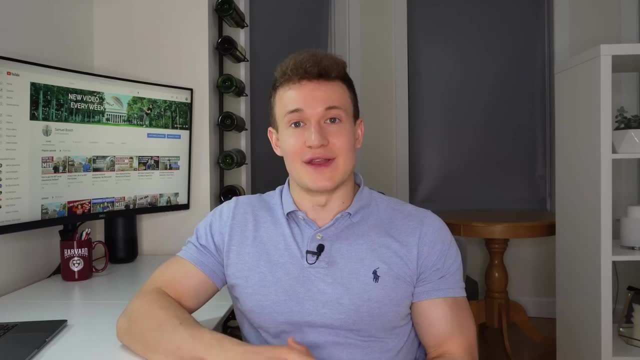 fix more cars with a $20 toolbox from Amazon than I would be able to do with a $100,000 mechanic shop. Let me give you an open-ended question that captures the essence of mathematical intuition really well. What is the total length of all the tunnels of London's public transport system? 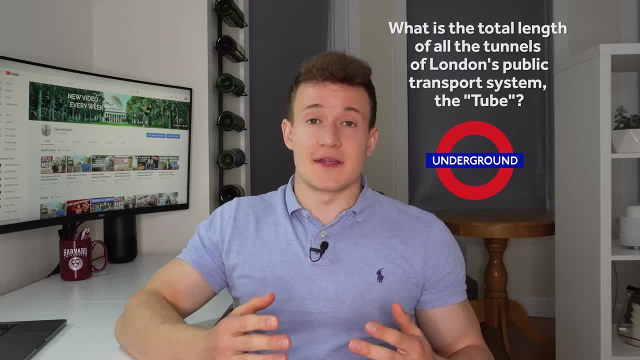 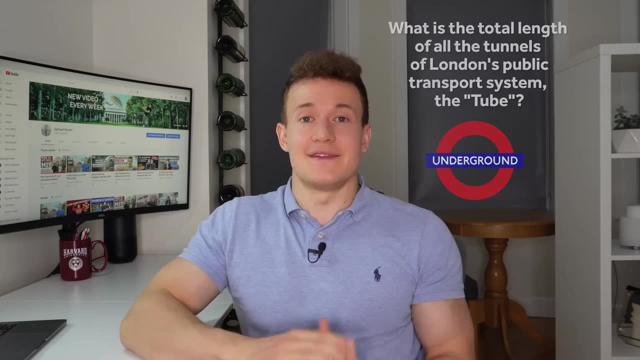 the Tube. This is a slightly simplified version of a question that I was asked during the first interview round for my aforementioned internship that later paid me $15,000 per month as an 18-year-old student. The worst way of solving such problems would probably be like preparing. 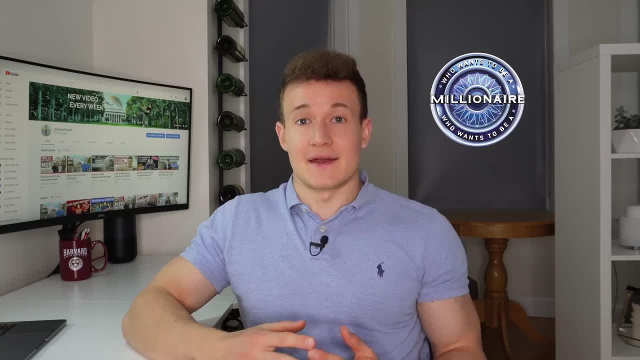 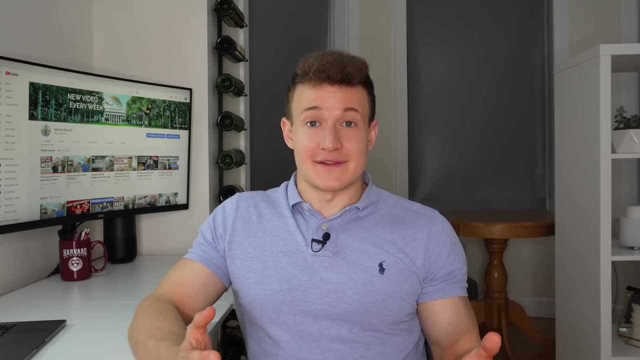 for the TV show called Who Wants to Be a Millionaire. That is just memorizing random facts about everything and hoping that one day some of these facts will actually be useful for something. Memorizing some things may be really good for your general knowledge, but it won't. 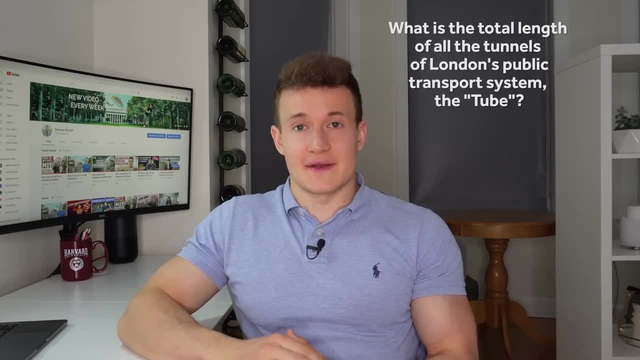 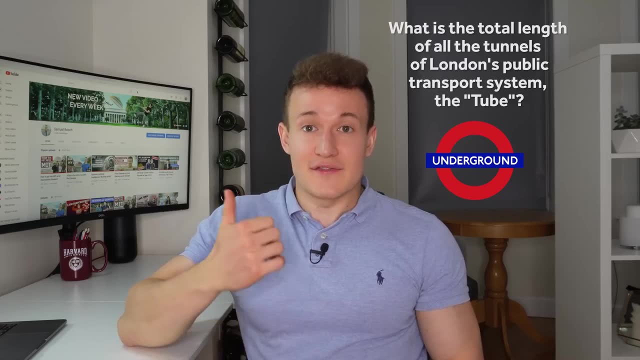 really well. What is the total length of all the tunnels of London's public transport system, the Tube? This is a slightly simplified version of a question that I was asked during the first interview round for my aforementioned internship that later paid me $15,000 per month as an. 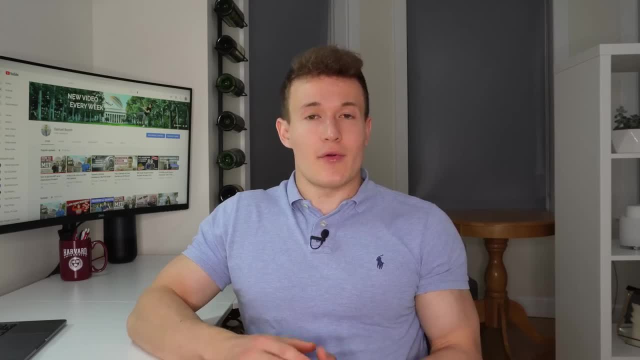 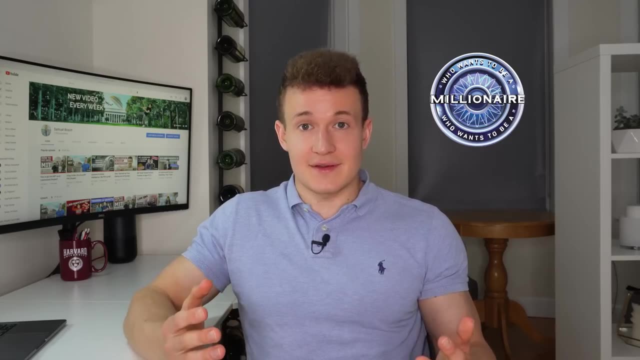 18-year-old student. The worst way of solving such problems would probably be like preparing for the TV show called Who Wants to Be a Millionaire. That is, just memorizing random facts about everything and hoping that one day some of these facts will actually be useful. 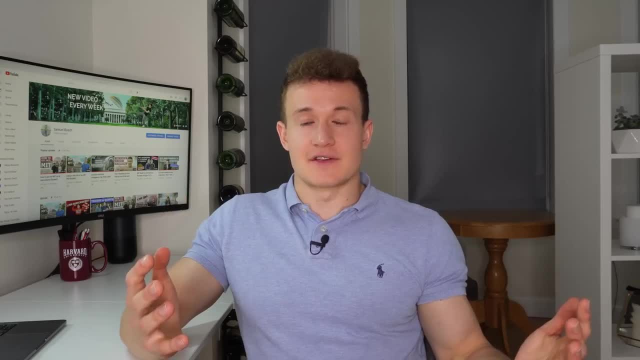 for something. Memorizing some things may be really good for your general knowledge, but it won't really get you far Because, honestly, what were the chances that you would have actually thought about memorizing this specific fact, unless you actually live in London Instead? 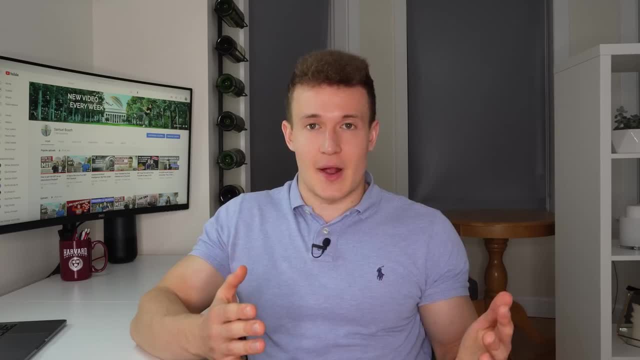 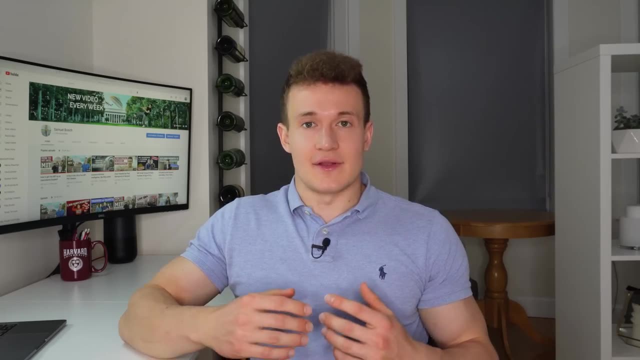 I want you to develop a great problem-solving strategy for attacking such problems with whatever weapons you have available to you at that moment. Instead of just guessing, I want you to explain to me how you would calculate the length of these tunnels by using only information that is available to you and without using a calculator. 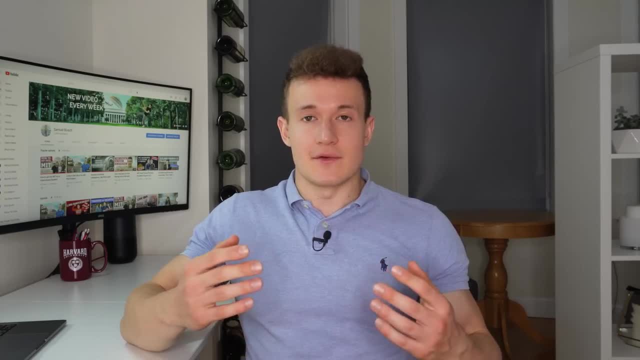 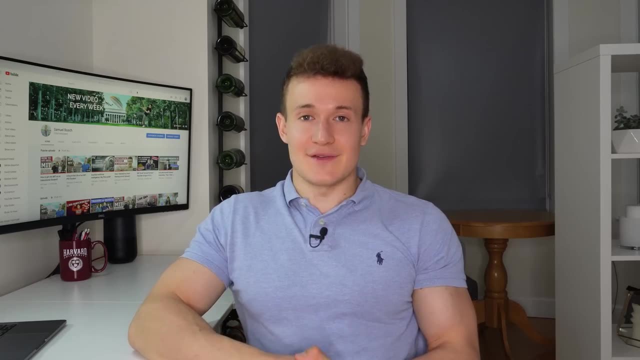 There are many ways to solve this problem, so I encourage you to describe your solution in the comment section down below and once the video hits 100,000 views, I'm going to pick my favorite solution and send the lucky winner a $50 Amazon gift card. If you're curious about 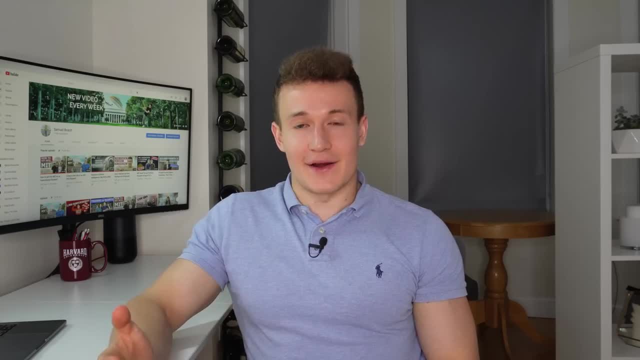 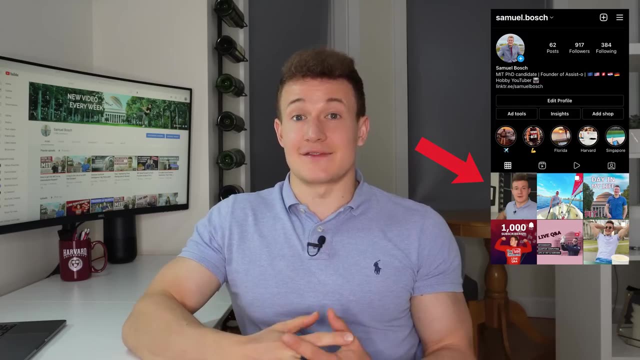 how I solved the problem during the interview process. I made a video about it and put it to my Instagram account. so feel free to follow me on Instagram and have a look at the video And, while you're there, feel free to send me a nice message and let me know if you. 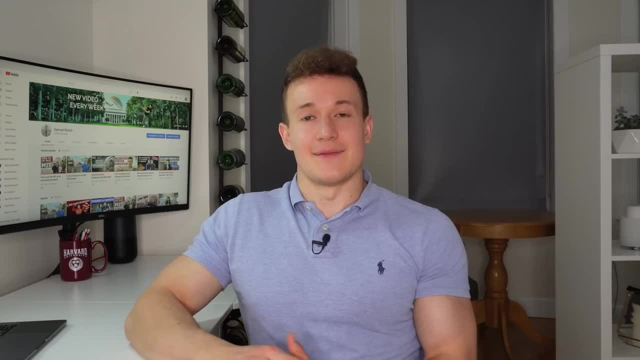 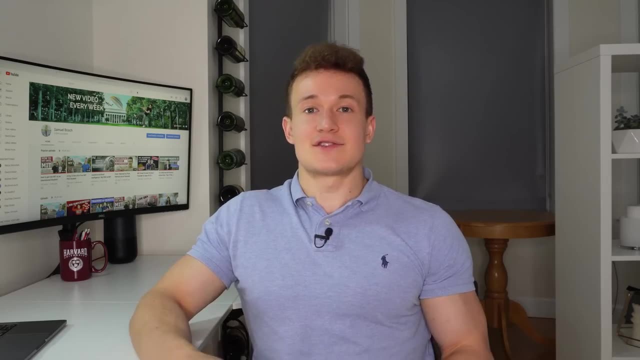 enjoyed this video. Special shout out to my friend and colleague at MIT, Emily Mu, who helped me prepare this video. If you want to hear more from both of us about math competitions and interning on Wall Street, you can check out our podcast episode over here or, if you want to. 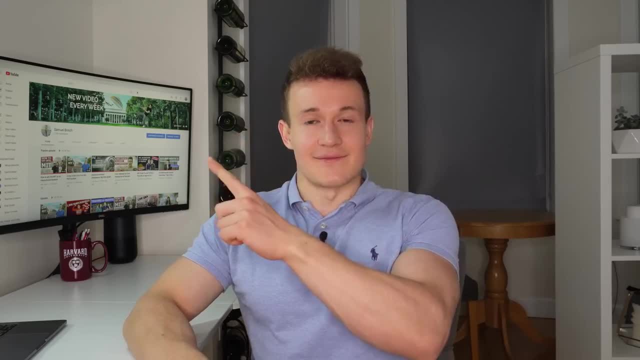 hear a video specifically about this internship. you can check it out over here. Thank you, guys, so much for watching. If you enjoyed this video, please give it a thumbs up and you can subscribe to my channel over here. I'll see you next time. Bye-bye. 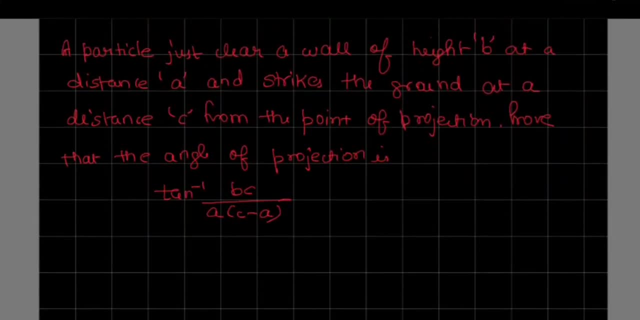 Hello and welcome to Ganesh Institute channel. So today we are going to discuss about mathematical modeling and in that too, how we can focus on the angle of projection. So let's have an explanation with the help of example. If you see here, this is your question, which.